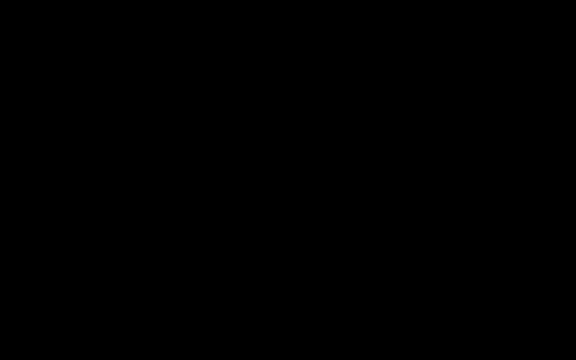 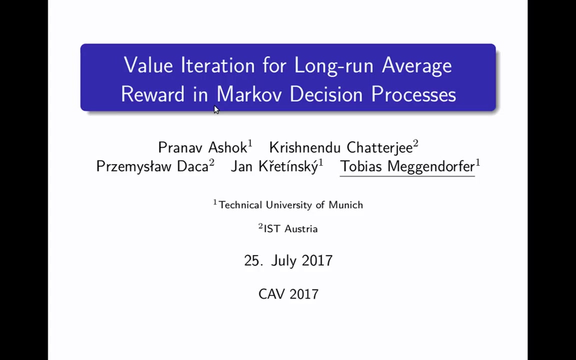 The last talk in this session is given by Tobias Meggendorfer on value iteration for long-run average reward in Markov decision processes. Okay, thanks for the introduction. This is joint work with Pranav, who's here in the audience, Krish Przemek and my supervisor, Jan. Let's jump right into it, because lunch 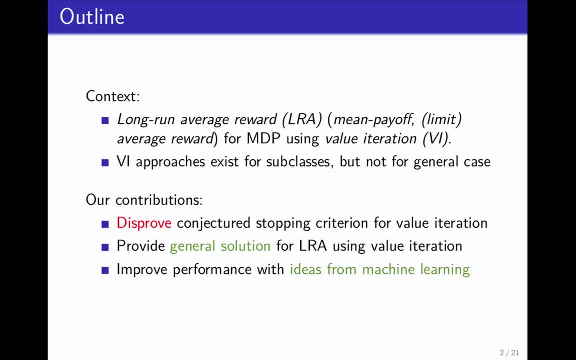 is coming close. First, I'm going to tell you about what you have to expect and why you should pay attention. So what we're trying to solve in the paper is the problem of long-run average reward on MDPs using value iteration. Some of you may know long-run average reward under the 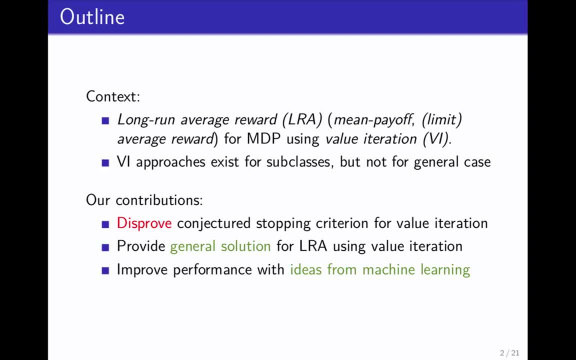 name of mean payoff or limit average reward, and there exists a gazillion of names for it. So, and it's also actually a quite old problem, but it turns out that value iteration approaches actually only exist for subclasses but not for the general problem. So we just try to. 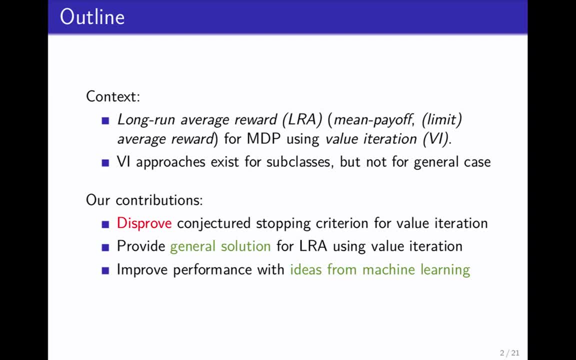 tackle that. So what we did is we disproved. we have disproven actually a conjecture made by Putemann like 20 years ago, related to that. We provide a general solution and we use ideas from machine learning to get a drastic performance increase while still maintaining accuracy. Okay so, 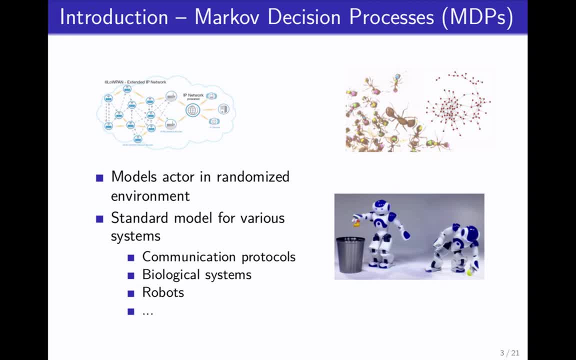 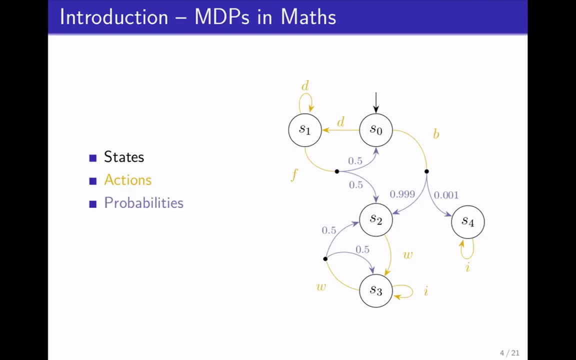 first introduction: MDPs- probably most of you know them, Standard model for actors in randomized environments. How do they look like in math? I hope yeah, one can see this. They have states In the states. you can choose an action and then 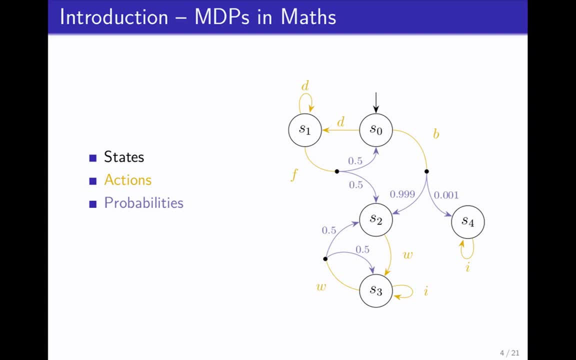 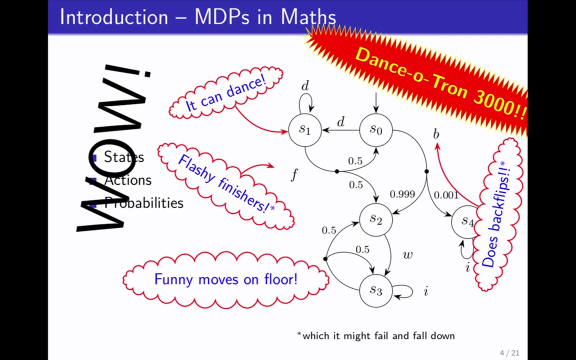 they. with some probability they take you somewhere. On the right side you see the toy example that will accompany us through the talk And actually it's quite literally a toy example, because it's the accurate model of the Densertron 3000 made by TUM Industries. 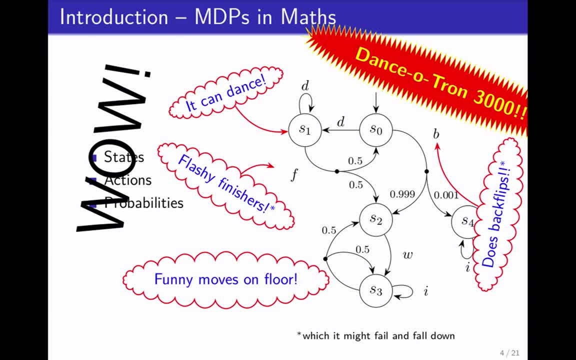 And it can do various things. So it's a small robot designed for dancing and entertaining people, and so what it can do is, well, it can dance, And then it goes to this dancing state and dance for you, And when it finishes dancing it does a super cool move. that's. 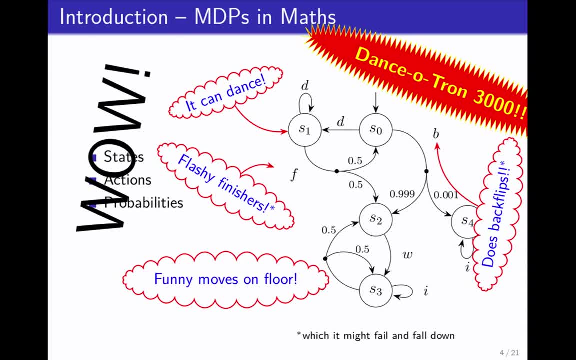 really impressive. It can also do back flips from the starting state And well, so the people were actually pretty lazy when implementing it. when it succeeds doing the back flip and then it kind of does it, And then it's kind of like is it going to be okay? And then it's like he's got it And then it's like it's not okay, but it's going to go away. So I think this is a really good example of how you could use it. I think this is a good 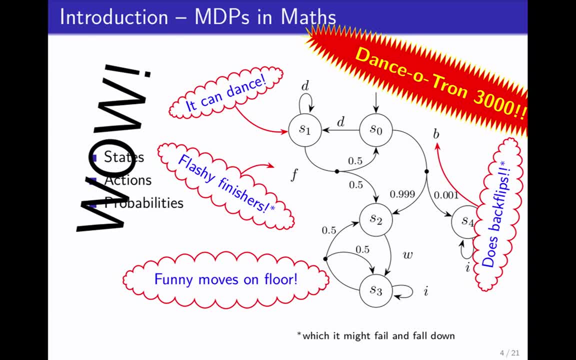 way of doing this. Yeah, Okay, Excellent, All right, Excellent, flip. it just stands there. Why were they lazy? Because most of the time the thing tries to do the back flip and just falls down to the ground and can't stand up. The same with 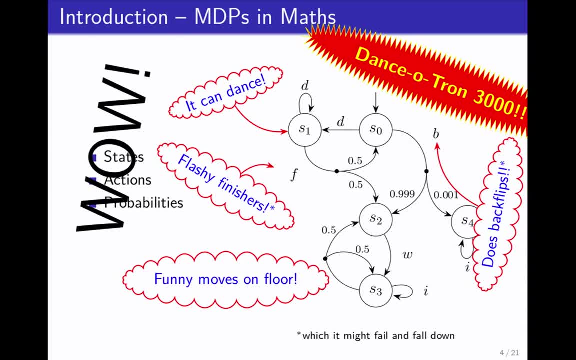 this: when it stops dancing, it might fall down and then it lies on the ground and the only thing it can do is kind of wiggle its hands. They were too lazy to implement the stand up routine, so that's about what it can do. 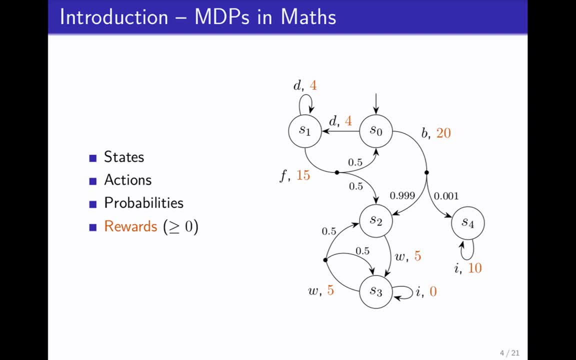 The next thing we add to MDPs are rewards. In this case, it will be my personal entertainment when watching the robot doing its things. When it's dancing, I'm kind of okay with it. When it does its flashy finisher move, I'm super impressed. Well, how can it do that? 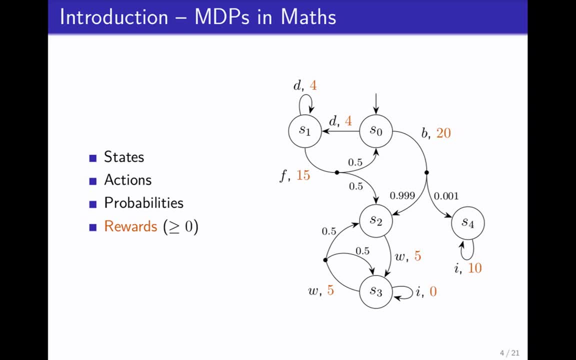 The back flip is just permanent amazement. If it tries it, I'm pretty impressed already, and if it succeeds in doing it I'll be eternally impressed. This is the biggest reward you can get in the long run here. If it's fallen to the ground and wiggles around its arms, then I find that pretty funny. 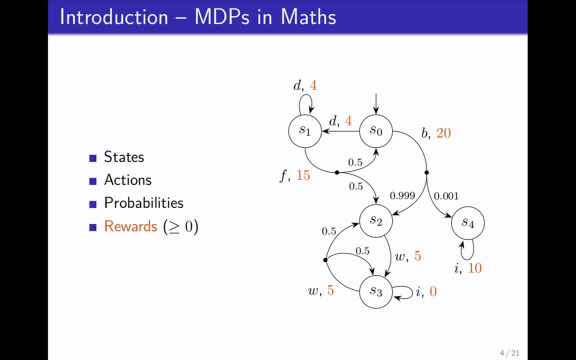 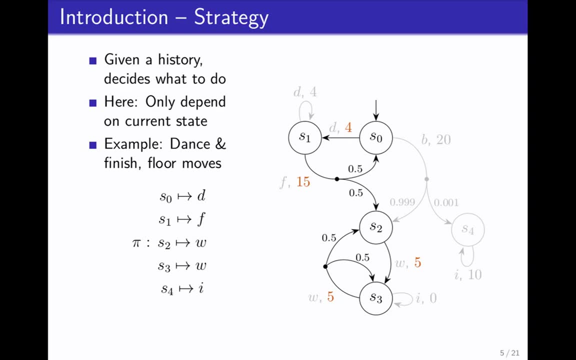 Just imagine a tortoise lying on its back and wiggling its arms. Pretty funny, I think. What's the next thing we need? We need strategies. We've seen that already- also named schedulers or something. It basically tells you what the thing does. Just imagine the program that. 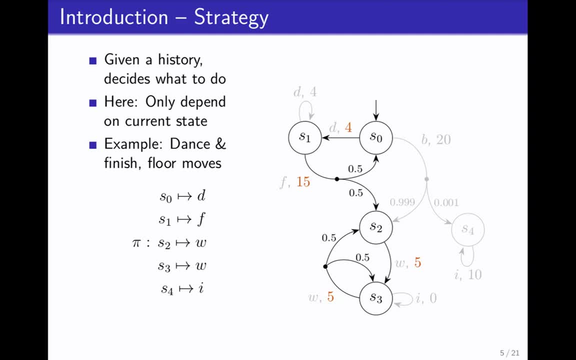 governs what the robot does In the talk. here we'll only consider state-dependent actions, state-dependent strategies- sorry. that basically are strategies that tell you, for each state, what I'm going to do. As an example, consider the strategy that tells you: start dancing, then immediately. 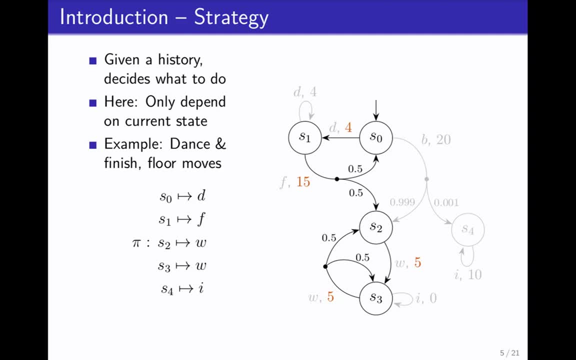 stop dancing and if you're on the ground, then do your thing. Then it kind of looks like this: I've grayed out all the unimportant stuff And when we completely remove it, hey, this looks kind of familiar. This is a Markov chain. 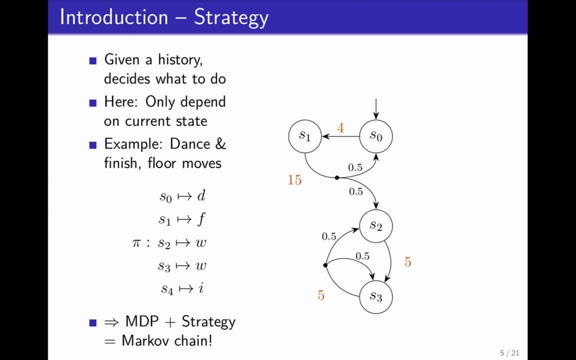 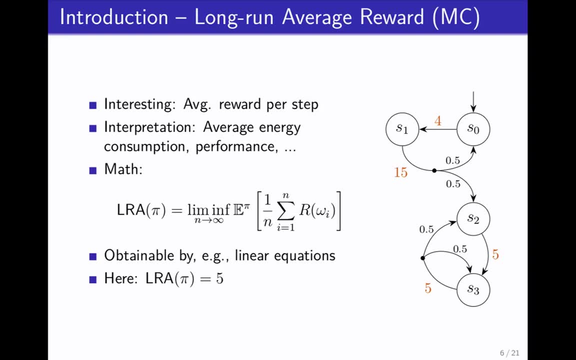 So what do we have? If we have an MDP, add a strategy to it, we get a Markov chain, And we know things about Markov chains. So for Markov chains, there also is this concept of long-run average reward, and it's quite. 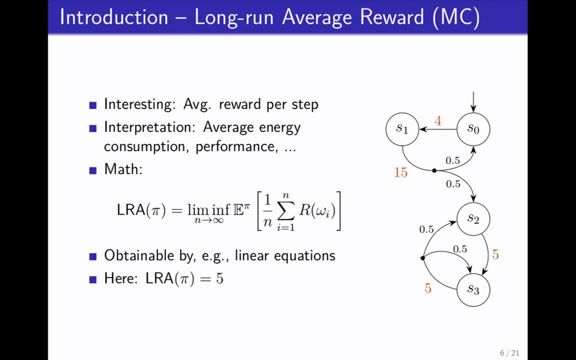 literally the expected reward you get in the long run. So it has an interesting interpretation. You can think of it as average energy consumption, some kind of performance metric, my average enjoyment or entertainment while watching this robot do its particular program. Okay, so here's the math. I'm not going to go into that. It's known how to solve this. 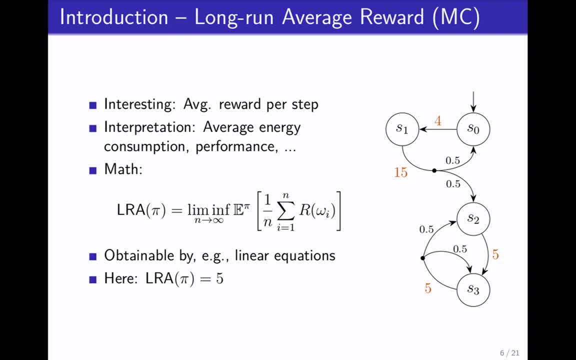 You can do linear equations whatever For this particular strategy. notice that eventually the robot will fall down on the ground and then do its floor moves, And so basically we get five reward on average. Okay And the like. the finite prefix doesn't matter because we only look at the limit. 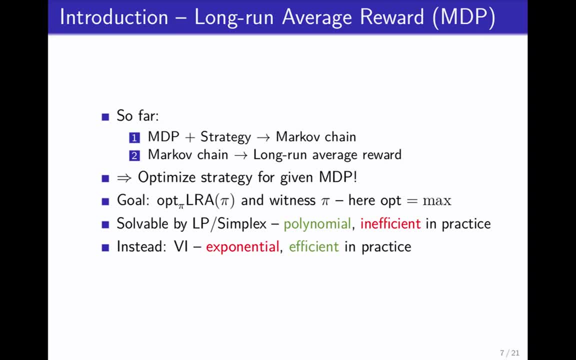 Okay. So what we've seen is we have an MDP and a strategy, We get a Markov chain. If we have a Markov chain, we get this long-run average reward thingy. So in a more abstract sense, we take something, we take an MDP, we throw something at it, we get out a number We can. 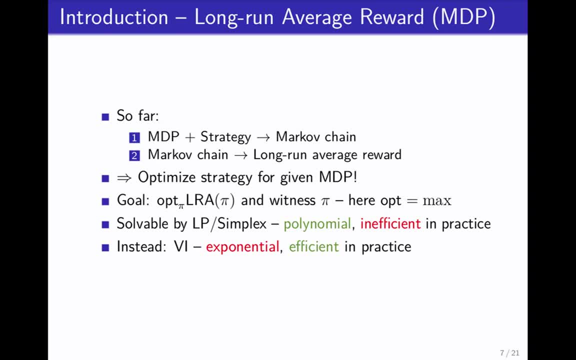 optimize this. So that's what we try to do. We try to find an optimal strategy which optimizes the long-run average reward. For the sake of simplicity, we'll only consider the reward maximization, But you can also do it with minimizations- completely the same. 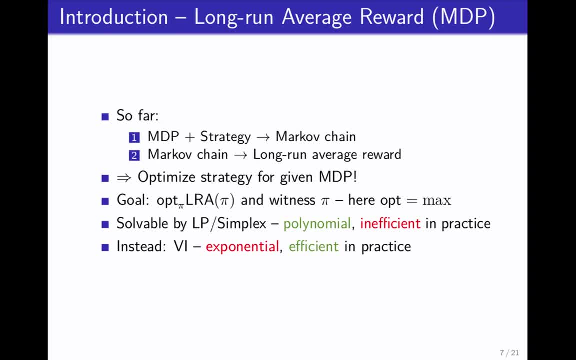 Okay, You can solve that by posing a linear program and then running simplex on it, which has polynomial time in theory, But in practice it just doesn't work for anything. So what you can do is use dynamic programming approaches like value iteration, which is like takes. 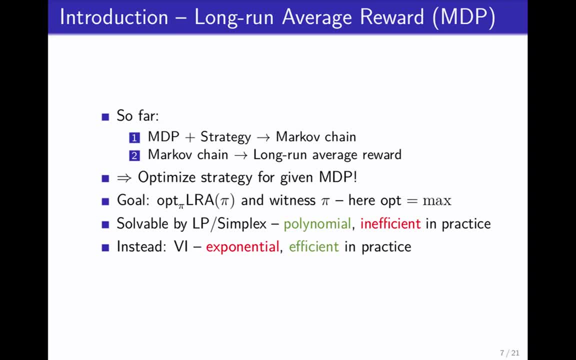 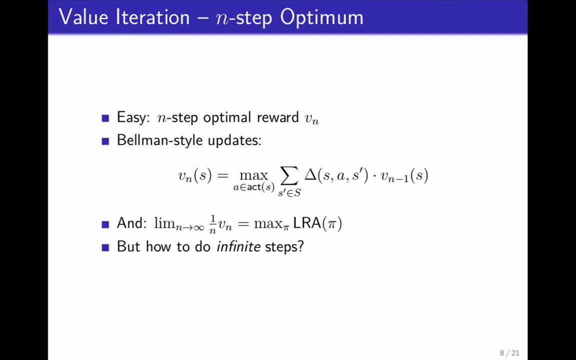 an exponential amount of steps in the worst case, But in practice it's just way faster, Okay. So how does it work? What's quite easy to get is the n-step average reward. You literally just do Bellman-style updates. And what's also quite obvious, I guess, is that if you 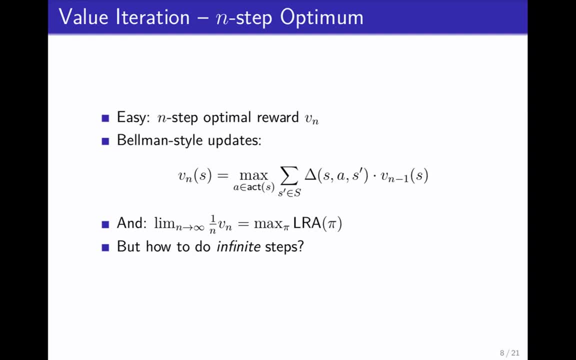 just average this n-step optimal reward, Then you get the n-step average reward. Okay, So now to get the long-run average reward, we just need to do infinite steps. But yeah, empirical data suggests doing infinite steps takes quite a long time, So we need to come up with something else. There actually is. 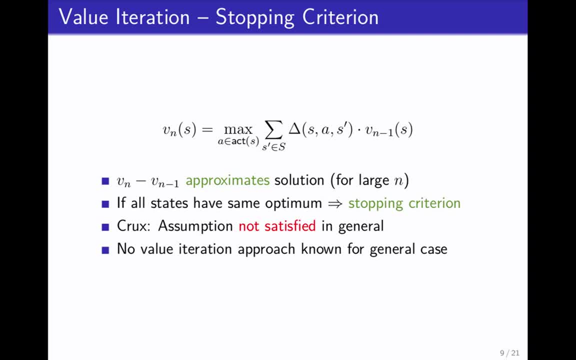 another thing that a stopping criterion that makes this work, that basically tells you: oh, I have these values And now I know that, well, I'm maybe not exactly at the solution, But you're like arbitrarily close, So we can kind of get an epsilon optimal solution from finite iteration. 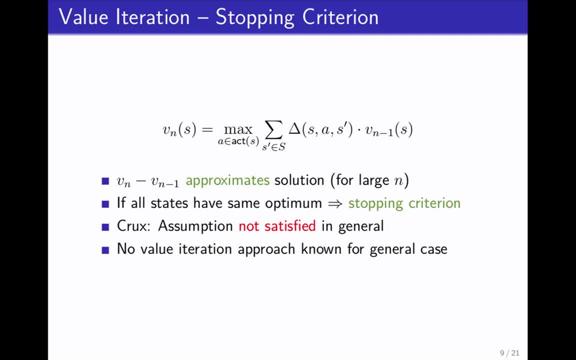 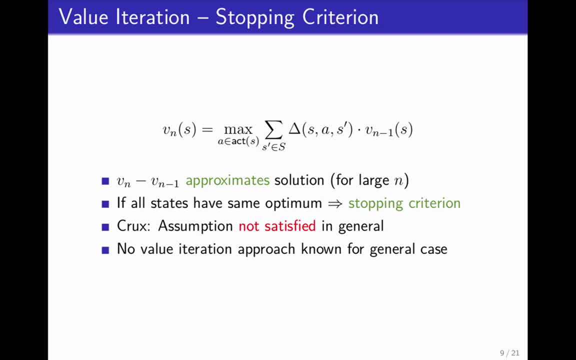 So now, if we have the same stiffness, we don't need to do infinite steps on this now. Yeah, This is also where the disproving conjecture comes in. There was a conjectured stopping criterion for the general case, But unfortunately it doesn't work, So we don't have a value. 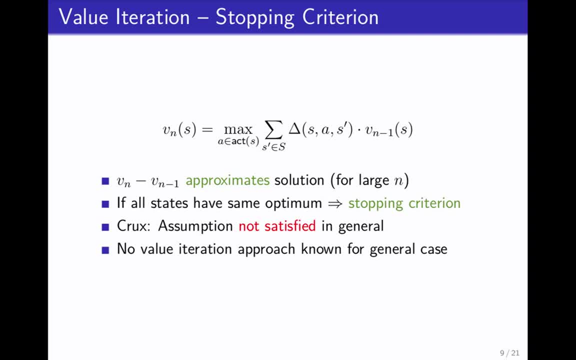 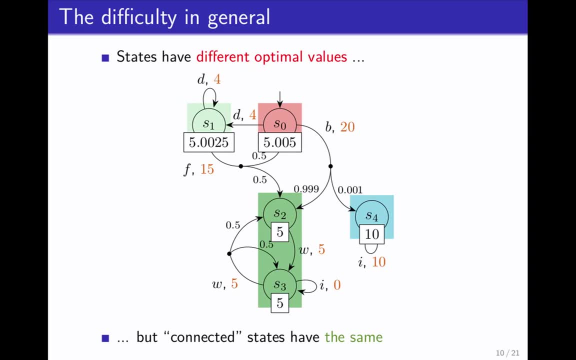 iteration that solves this problem in the general case. As an example, let's just go back to our yeah to the robot. We see that, yes, indeed, different states have different optimal values. So, for example, here this idle state after: 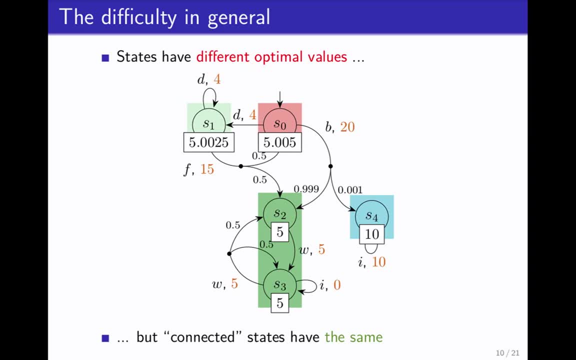 backflip is conform. So this is where this problem comes in. Let's go back to our has an optimal value of 10, because here you get 10 on average. Down here, when it's on the floor, you just get 5 on average. 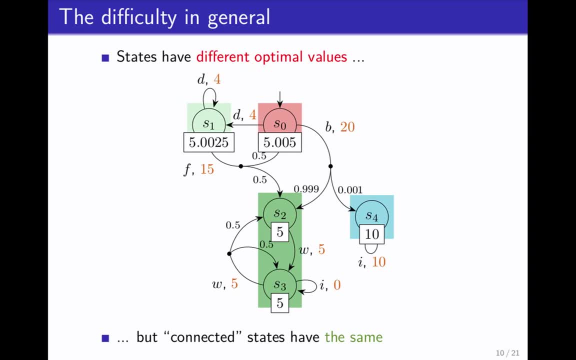 So, yeah, you have different values, But the thing you can observe is that states that are kind of connected have the same optimal value. So these two guys here have the same optimal value. Why is this the case? This is basically the key concept to the solution here. 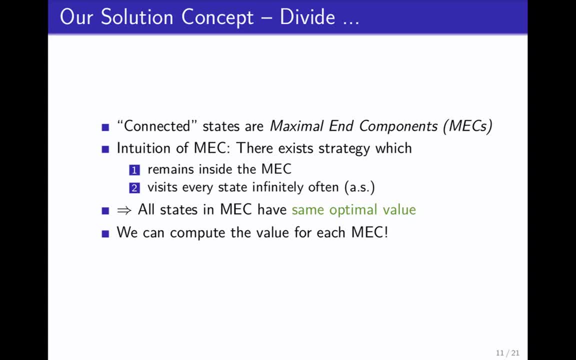 So these connected states are actually just MACs. MACs are parts of the state space in which you can remain for infinite time, if you decide to do so, in a nutshell, And all the states in the MAC have the same optimal value, which is, I think, quite easy to see. 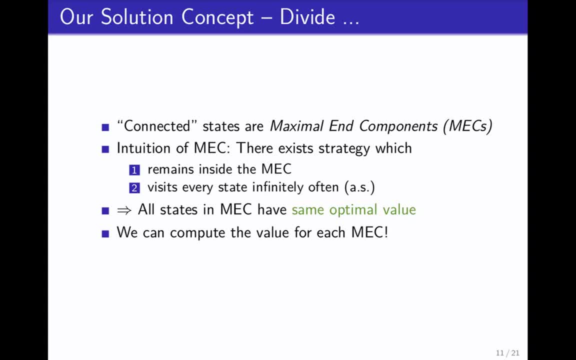 because suppose that some state has some optimal value, then by definition of a MAC you can't just go there in finite time, almost surely, And then do whatever needs to be done to get the optimal value there. Okay, So now we know, oh, we can actually compute values for each MAC. 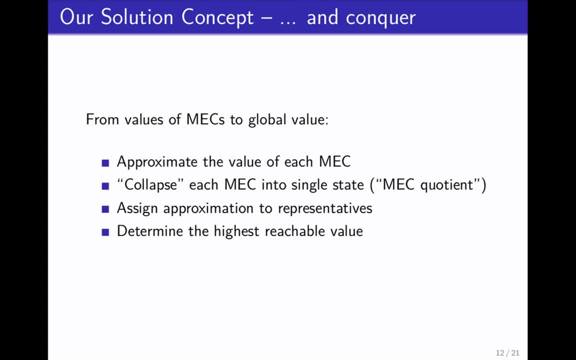 This isn't the whole solution, but half of it. What's only missing now is: hey, how can we go from we have values for each MAC to what's the global value? And well, we came up with a simple solution. 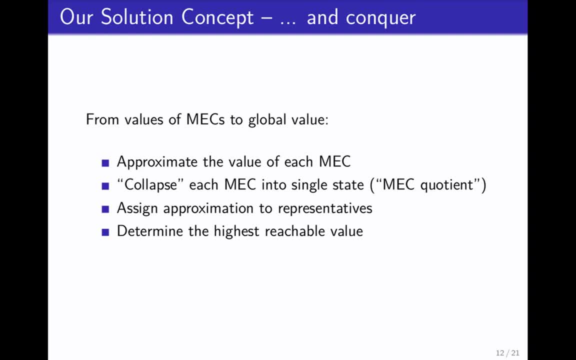 and that is to we first approximate the value in each MAC or determine the value of each MAC, then collapse all of these MACs into representative states and then solve a weighted reachability problem, which I'm going to explain again with the example. 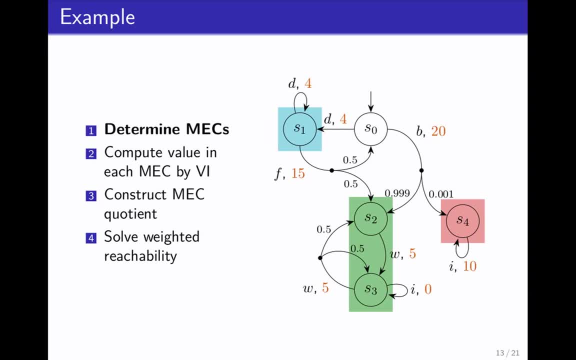 So what are we doing? We determine the MACs, We compute the values in each. Okay, so up here we have a value of four, because the best you can do while remaining in here is just, yeah, you can do this. 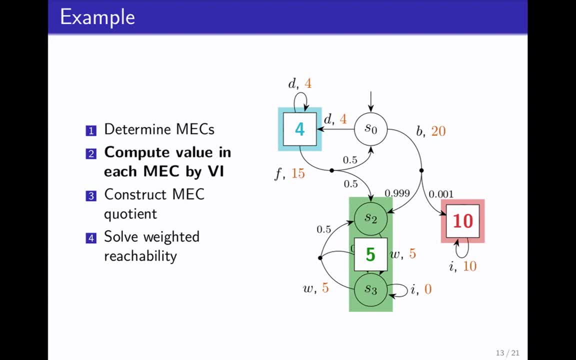 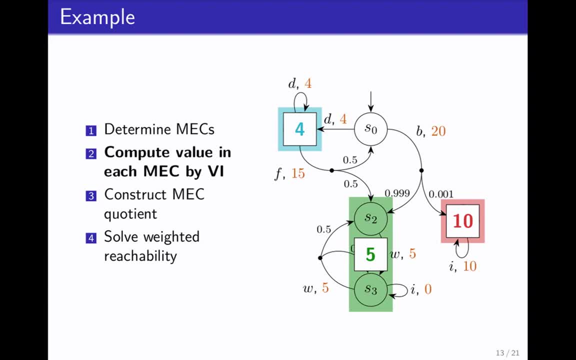 is just, yeah, having the five, Okay, Then we collapse them. This is a construction known as the MAC quotient. We have taken the existing definition and modified it slightly to, like, make things a bit more, a bit faster. But yeah, in essence you just collapse these MACs. 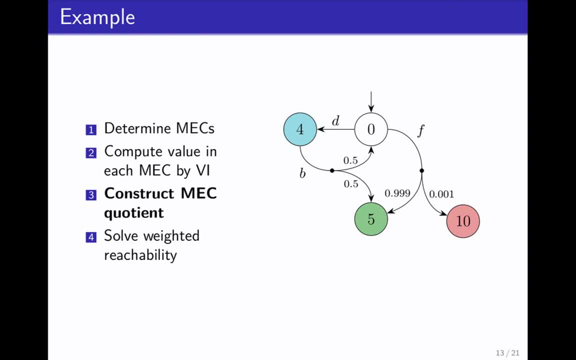 have one state representing them. give this state the value of the MAC, and then you try to compute weighted reachability. Weighted reachability in this context just means: well, what is the maximum value I can get to on average? So here we do that. 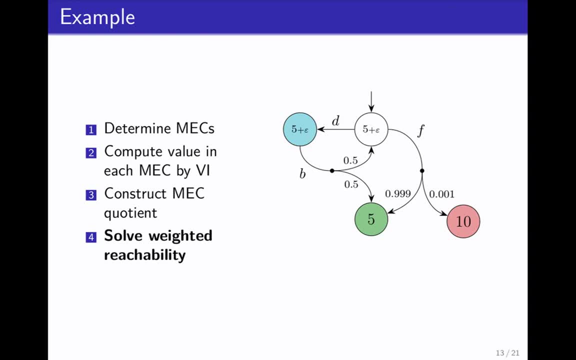 We see that, for example, this guy here, it had a value of four before, but it can actually go to five and something by actually stopping to dance- and there should be an F sorry- and trying to go over there to these guys. 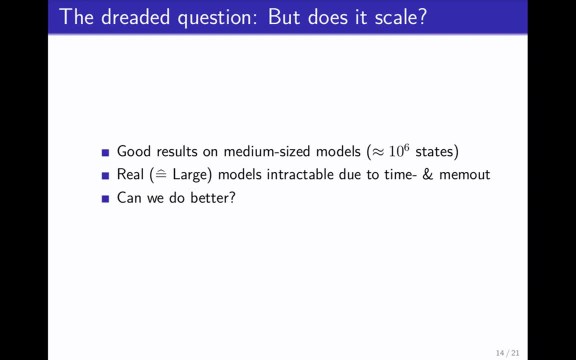 Okay. So when you look at this I think, oh yeah, there comes the dreaded question: does it scale? It kind of gives reasonable results on models with, say, a million or 10 million states, but real models tend to be larger than that way larger. 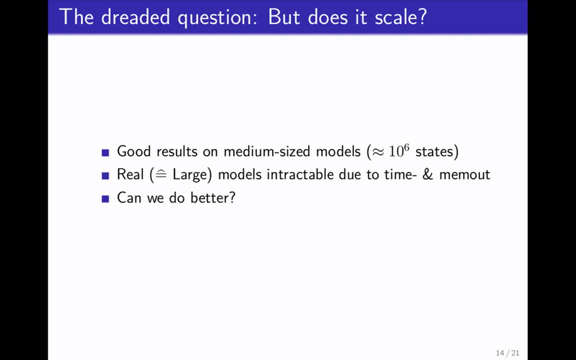 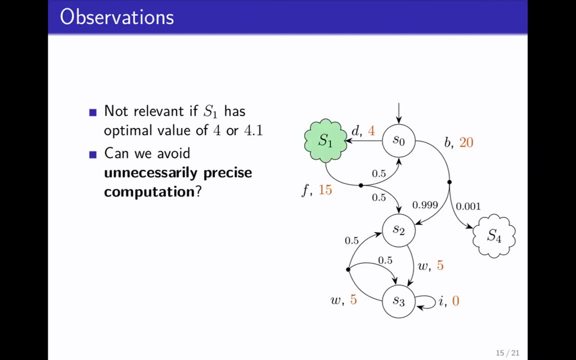 And they tend to be even too large to fit into memory. so we immediately get time or memouts. And now the question is: can we do better somehow? Okay, We made two observations. The first observation is that, consider: Tom Industries now released a new, improved version. 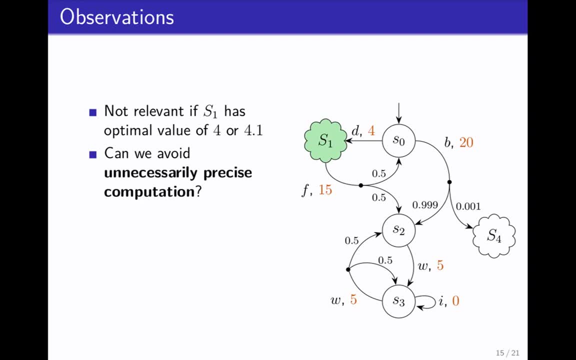 of the robot where the dancing subroutine is like really super advanced, and there are a million of states in there same, with they actually bother to implement what happens after the backflip, and there are 10 million states after there too. And the first observation is that 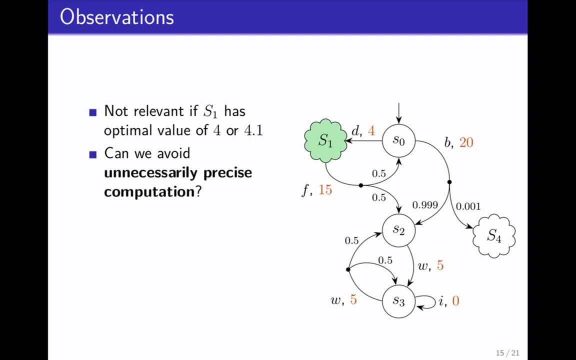 can we somehow get a bound on what's happening inside this dancing subroutine? It doesn't matter what's the precise value. So if it has a value on average reward of 4 or 4.1 or 3.9, it doesn't matter, because down here we get something better. 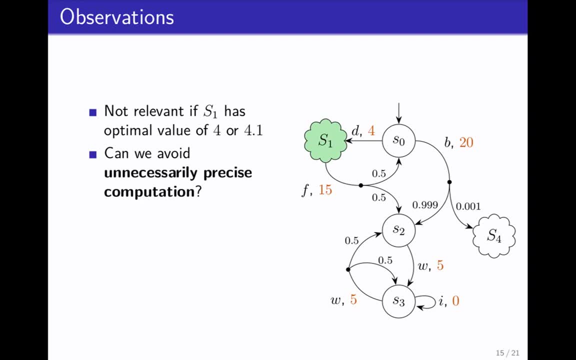 Okay. So the first question is: can we avoid unnecessarily precise computations? We don't need the precise value here. The second question is: well, what happens after the backflip actually really doesn't matter. It happens with so little probability that, if the precision we want to have is reasonable enough, 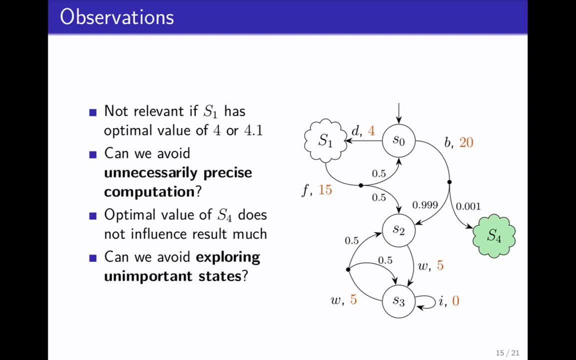 then we don't actually need to compute what's happening over there at all. So we don't need to look at the states at all, given that we have some kind of upper bound on the reward you can get. So if the user tells us, or if I say: 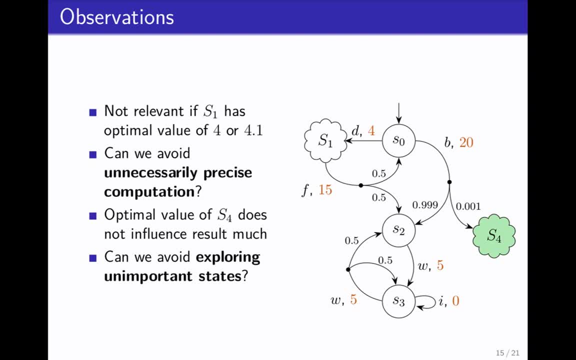 well, the most entertainment I can get is 20 or something per time unit or per step. then I don't need to bother to look at what's over there, because I can only get 20 at most. and it happens with such little chance that, yeah, why should I look at it? 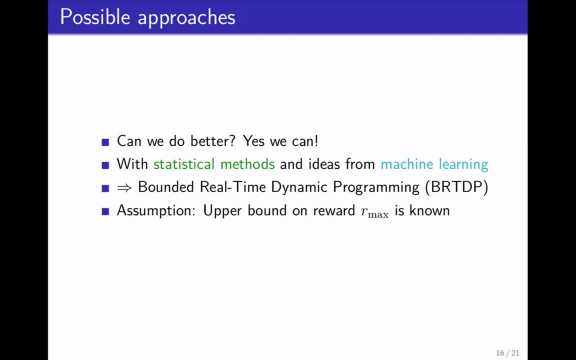 And so we made this observation and spoiler alert. yes, we can do this, And we're using for this statistical methods and ideas from machine learning. The idea is more or less described as bounded real-time dynamic programming. That was mentioned before already. 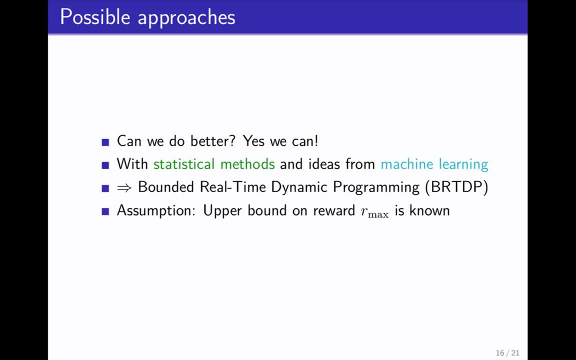 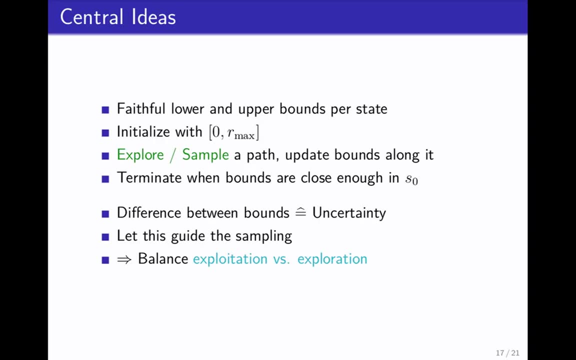 The only assumption that we make is that you kind of get an upper bound on the reward, which is, I think, a reasonable assumption. So what do we do We basically? we initialize lazily, we give all the states a faithful upper and lower bound. 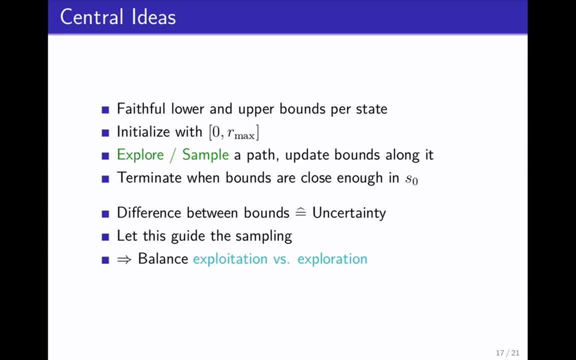 which is also related to the ideas presented previously. We just initialize it with zero and the given upper bound, and then we- yeah, this is where the statistical methods come in- We sample a path and then we somehow update the values along this path. 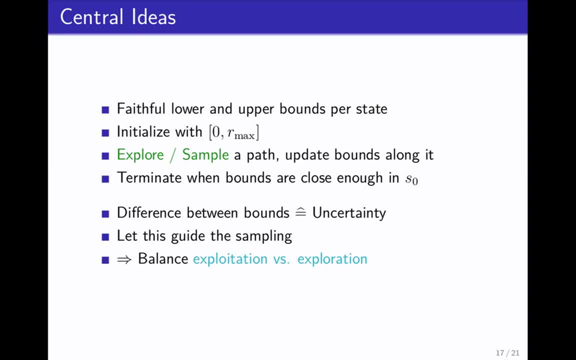 by a method I'll explain on the next slide And we'll just terminate when the bounds are close enough in the initial state, So basically where we want to know what the values are. Okay. so the difference between the bounds kind of give us a level of uncertainty. 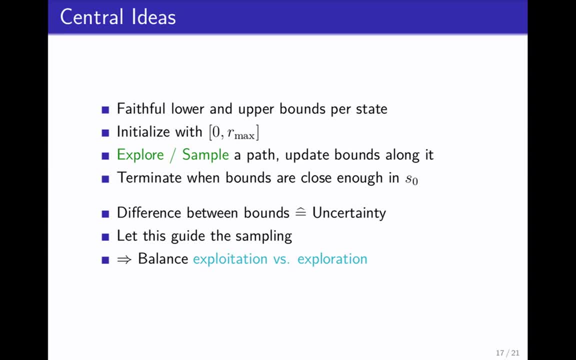 If a state has A high difference between the bounds, we have high uncertainty. If it's very, very close, like 10 to the minus 6, we kind of know what the value of this state is. And now the idea from machine learning basically just is. 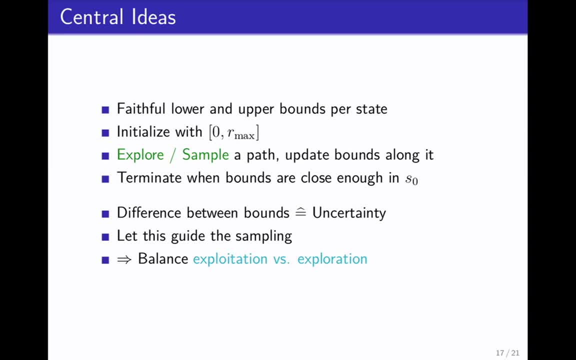 let this uncertainty guide our sampling, because this kind of balances, then, exploration versus exploitation. If we aren't sure about some region, we explore it. If we're sure that it's bad, we don't explore it. And now we have this bounds per state. 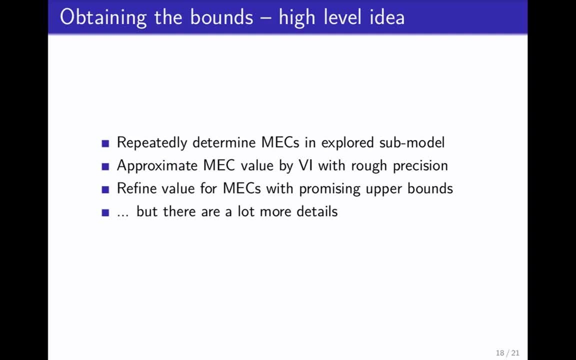 and we need to update them. The very high-level idea- this is actually where kind of the central part of the paper lies- is a bit tricky, but the high-level idea is that you sample paths. This gives you a sub-model, Basically. you haven't seen all the states. 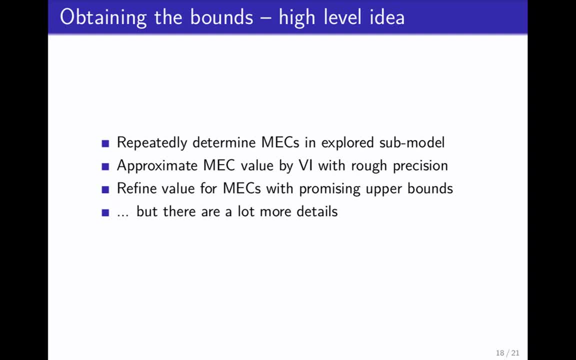 You just memorize the states you have seen so far In the sub-model, you repeatedly determine max, collapse them And in these max, you approximate the values using the previous approach. And Whenever the algorithm decides: hey, this region looks interesting. 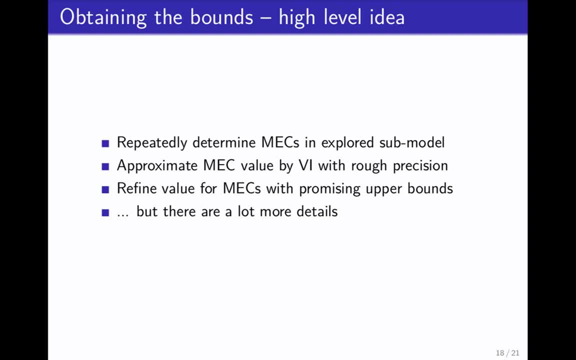 then you refine the values And Yeah, you kind of Yeah when the mech has promising upper bounds, But yeah, it's kind of tricky. so if you're interested in this, just look at the paper. I don't have time to go into that, unfortunately. 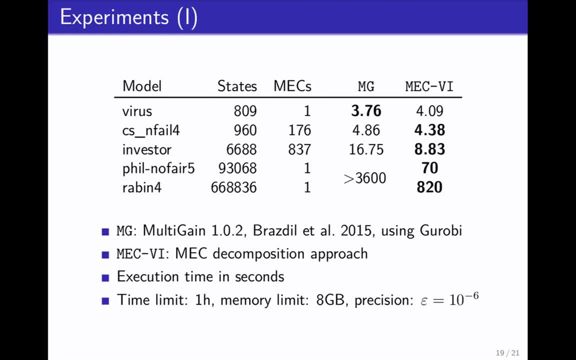 So yeah, Now that's the theory. Now I'll give you the numbers. The numbers are, I think, quite good. We compare to the only tool we found doing mean payoff, which is multigain. It's actually built for multi-objective multigain. 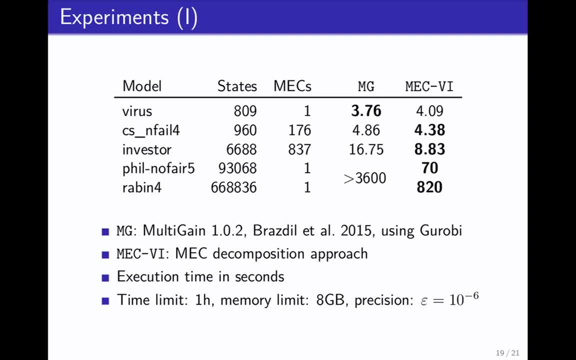 so the comparison isn't completely fair. But as you see here, we just completely beat it in any reasonable model And we also improved the implementation a bit to get these numbers down to more like, say, 50 and 80 or something. 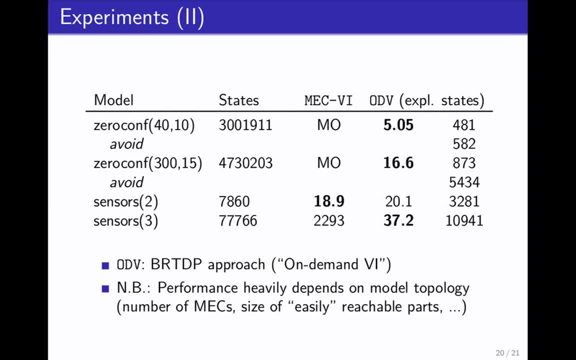 Okay, And now here comes the cool thing, This machine learning guided approach, which is we call ODV. It's an on-demand value iteration, And the most interesting model is the ZeroConf model, which has, in this instance, like 4 million states. 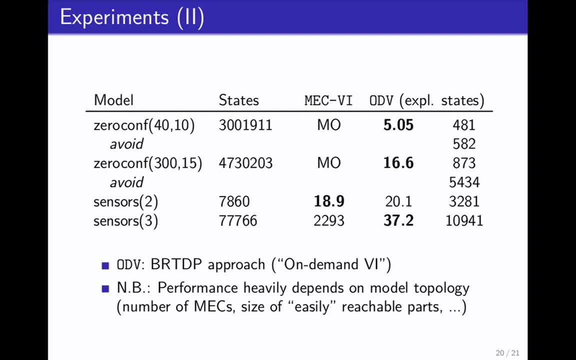 But to compute a value precise to 10, to the minus 6, we only needed to explore like 1,000 states of this million And, yeah, we needed 16 seconds to do that. In a new implementation we got this down to roughly a second or something. 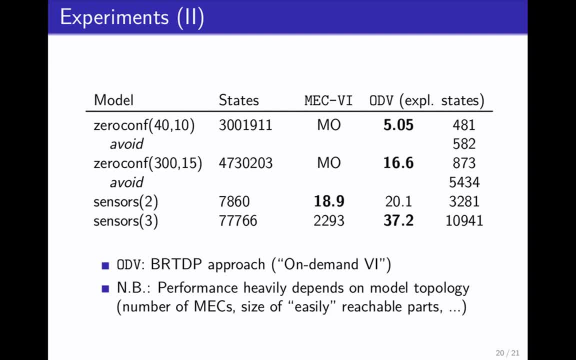 So it really works for some models. For other models it's the same as the previous approach. It just depends on the topology. If the whole region of the state space is interesting, you have to explore everything. There's no way around it. 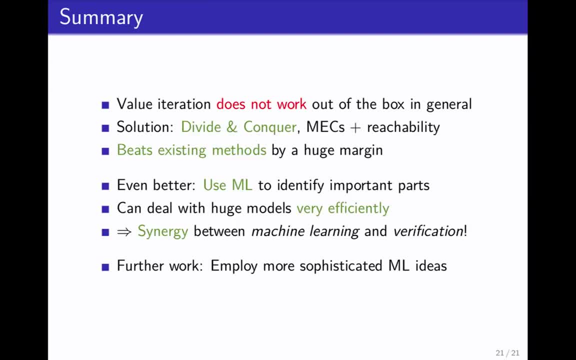 Okay. So, in summary, what have we done? We've shown that value iteration does not work out of the box. in general, We provided a simple solution, which is a divide-and-conquer approach. This already beats existing methods by a huge margin. 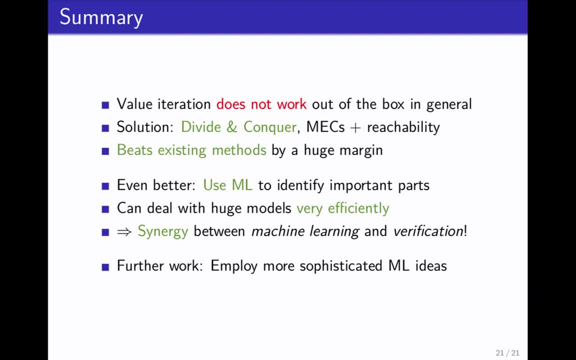 Even better. we use machine learning to identify important parts and then focus our computation on that. And this is kind of the key takeaway note I want to give in this talk is: you can actually use machine learning for verification without sacrificing precision. You just use machine learning in some way. 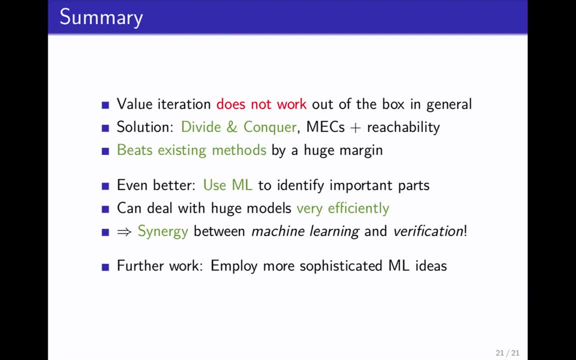 to identify the important thing and then do whatever is the right thing to do there. And well, further work, more sophisticated machine learning. I mean this is kind of a simple machine learning idea. They have that for a long time. Maybe we can use some kind of neural network. 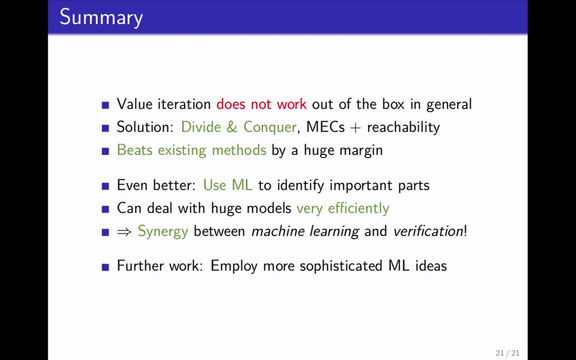 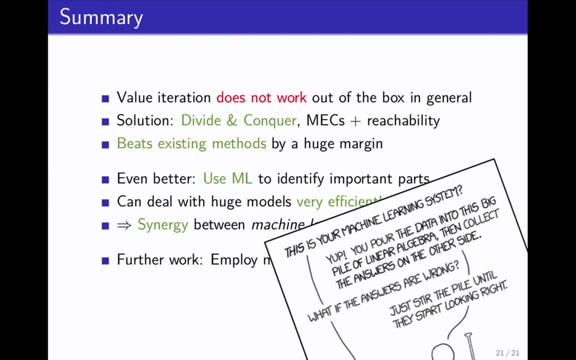 something to do. a bit more interesting stuff. Okay, That's all folks. So now it's time to ask questions or go for lunch, Your choice: Questions- Everyone is blown away. I was wondering about that dancing robot. So the reward for successful backflip? 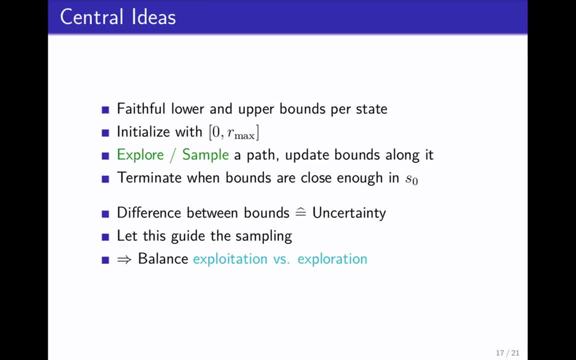 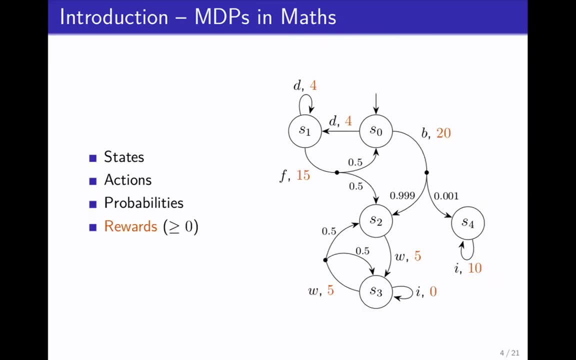 it was large, but it was not. Wait, Let me go back to the model, then we can point at it. Where is it There? Okay, It was large, but not by an order of magnitude compared to others. So what happens if it's by several order of magnitudes? 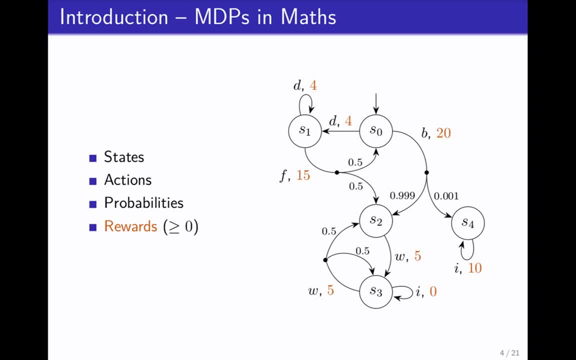 Which reward For doing successful backflip, Then yeah, basically, then you have to look at this option Like you have to explore it and say- or maybe you also just know that the upper bound on the rewards is very rough.